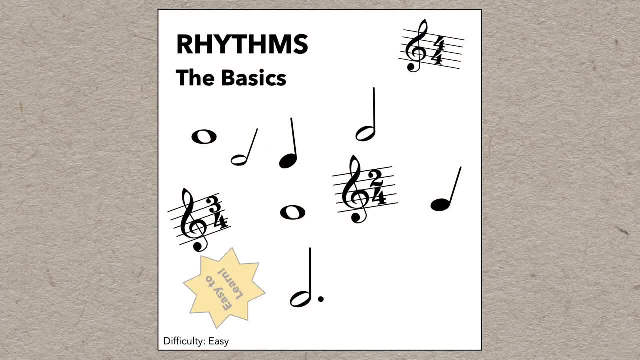 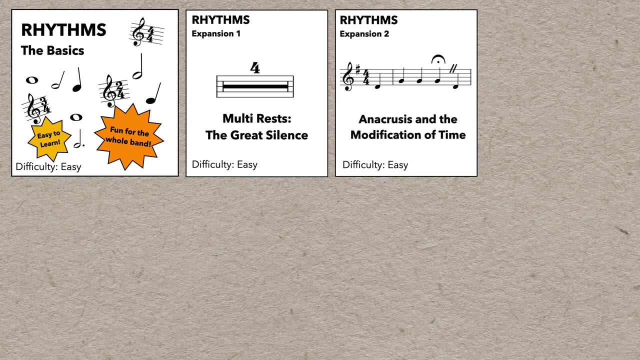 You can almost think of it like a board game. The basic rules are pretty easy and you can do a lot with a base game, But after a while you're ready for more complexity and you can even start adding expansions. Each one has a bit of a learning curve. 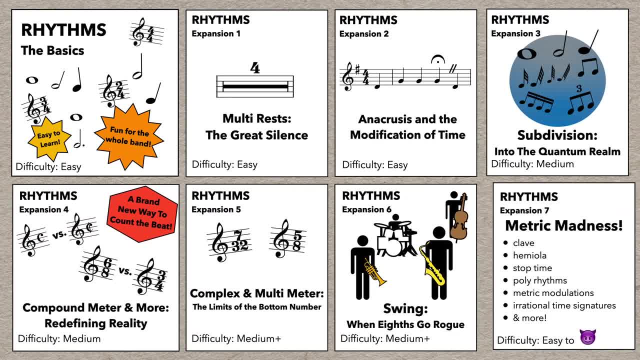 but it's manageable if you do it bit by bit And each installment really excels at its own level. So if you're a beginner you can do a bit of a learning curve expands the possibilities of the game. We'll be covering these three in this video. 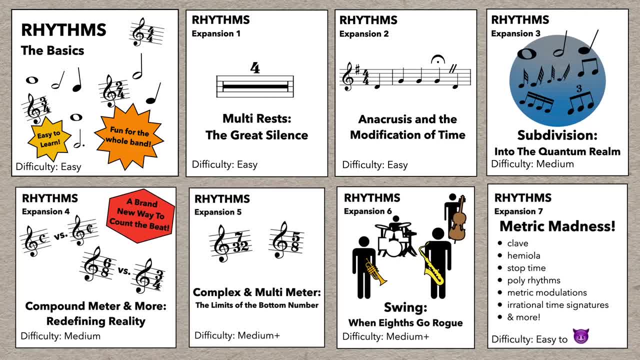 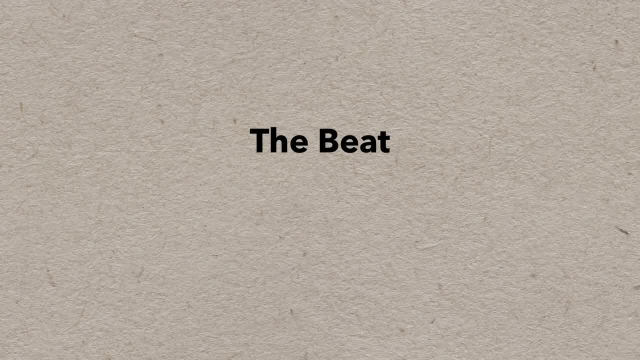 which will be plenty to get you started, And we'll save these other more advanced expansions for upcoming installments. So let's get started with the rules of the base game. The most fundamental concept to understandable rhythms is the beat, which is the basic underlying. 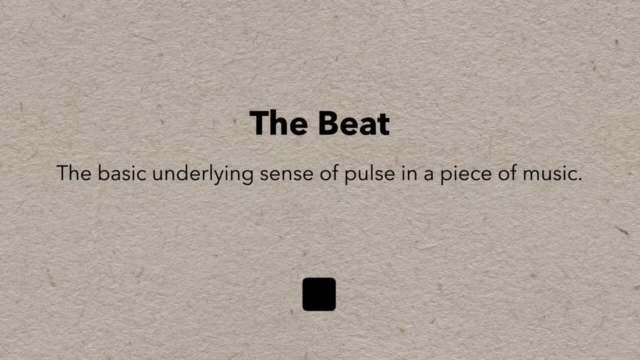 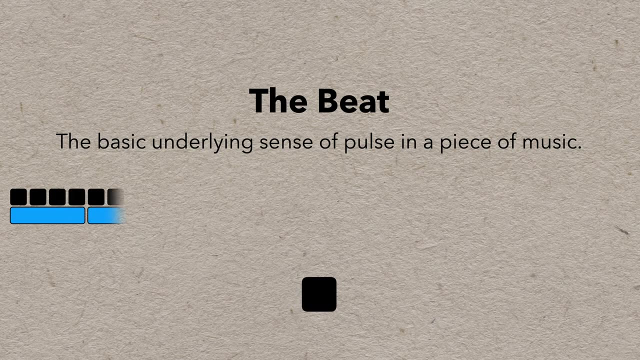 sense of pulse in a piece of music. Most of the time the beat just ticks along at a steady and consistent pace. There can be sounds that are longer than a beat or shorter than a beat. They can match right to the beat. 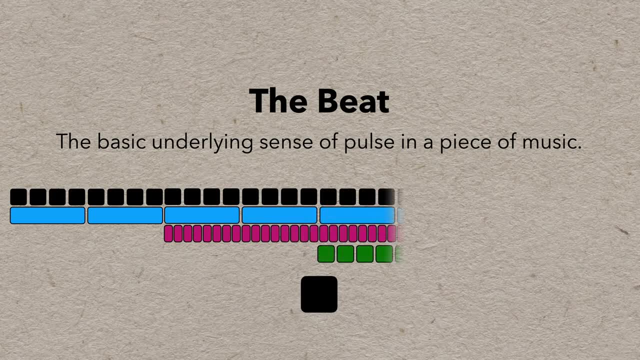 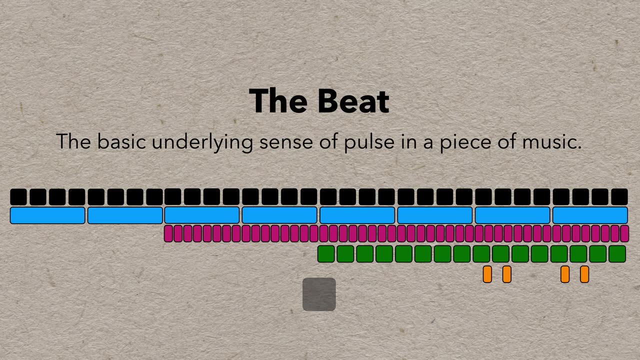 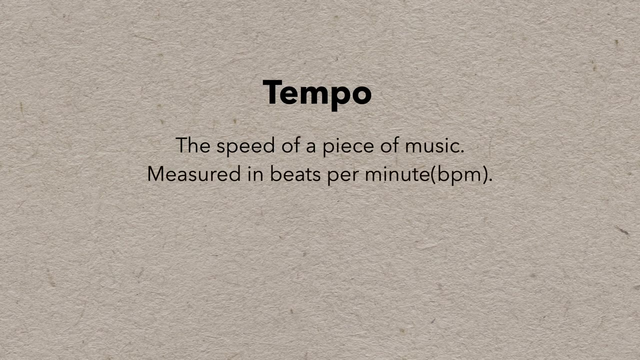 You can be up with the beat or be off the beat, But basically everything to do with rhythms is defined by its relationship to the beat. Tempo refers to the speed of a piece of music and is measured in beats per minute. This piece is at 120 beats per minute, which just happens to be. 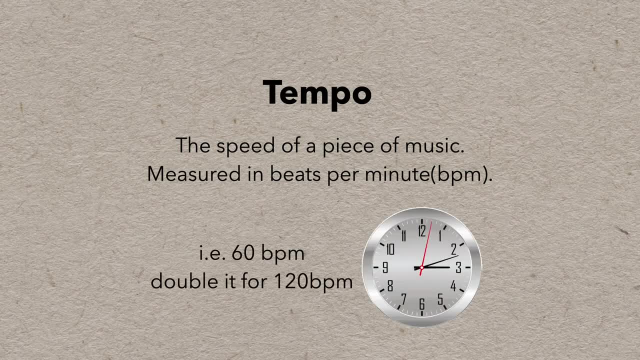 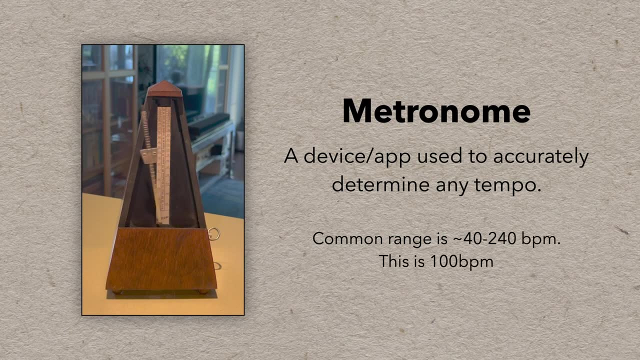 double a tempo that you're already probably very familiar with the second hand of a clock. You can also use a device called a metronome to accurately measure the beat. You'll find music tends to group itself into cycles of strong and weak beats. 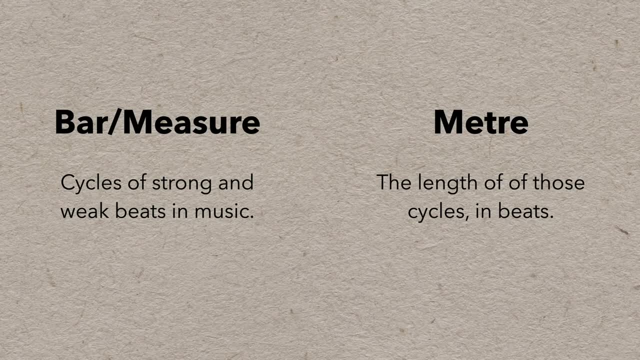 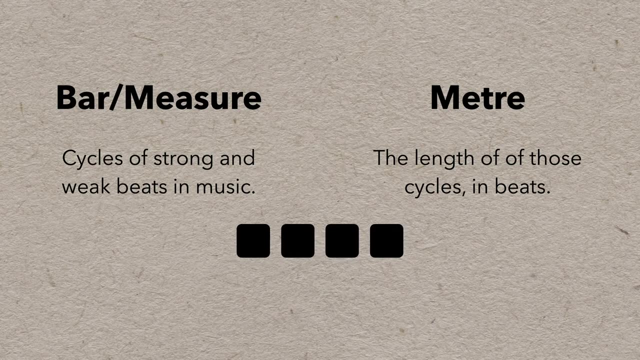 which are known as bars or measures, And the length of those bars is known as meter. You'll hear 4 beats per bar pretty often. It's an incredibly common meter across nearly every genre of music. It has a strong beat on one, followed by three weaker beats. 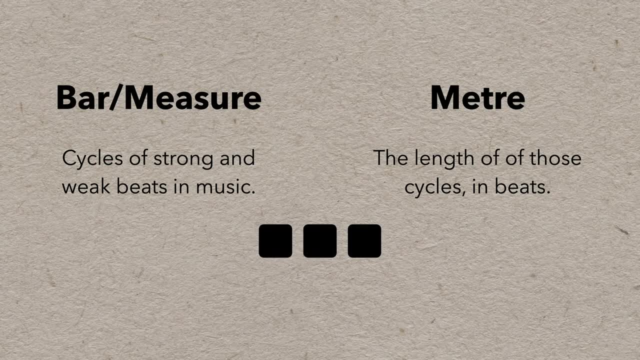 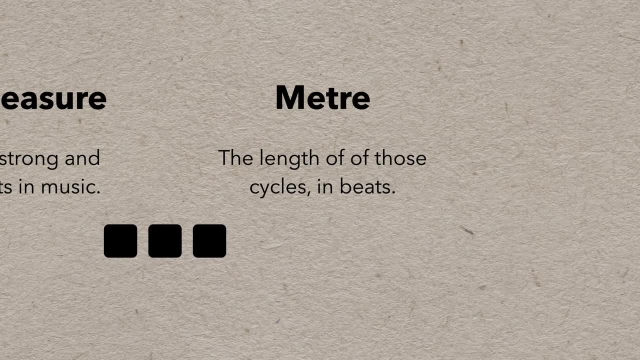 You'll also hear a lot of music with three beats in a bar, which has a strong beat on one followed by two weaker beats. You'll hear a lot of music with three beats in a bar followed by two weaker beats. Meter gives rise to a type of notation called a time signature. It consists of two numbers. 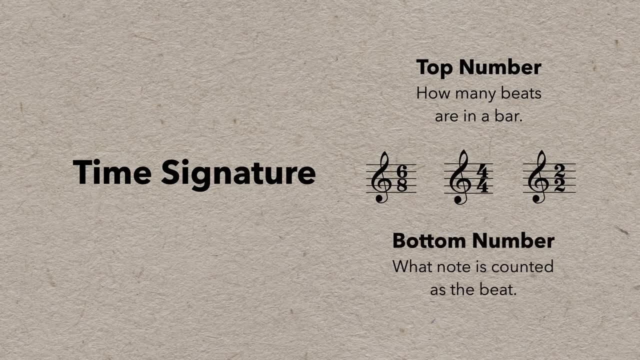 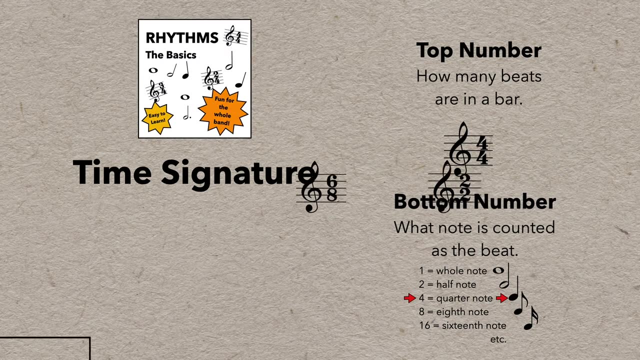 The top one tells you how many beats are in a bar and the bottom one dictates what kind of note is counted as the beat. For now we're only dealing with time signatures with four on the bottom, which means we're counting the quarter note, And that covers a ton of music. but we'll 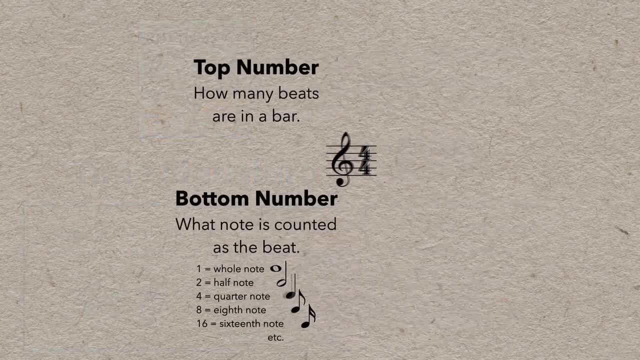 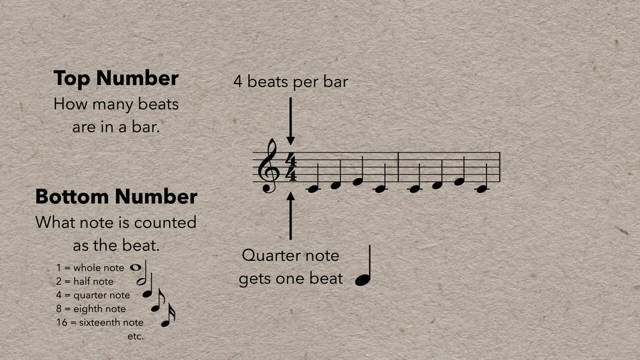 explore other options later on. So in 4-4 there are four beats in a bar and the quarter note gets the beat, And a couple of bars or quarter notes look like this: Each one gets the beat and they're counted for the beat they fall on. You can also have half notes which are two beats long. 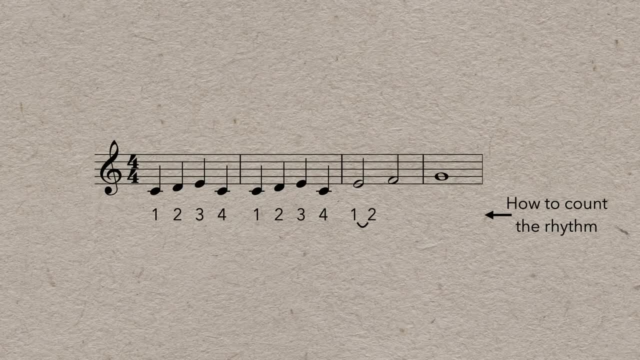 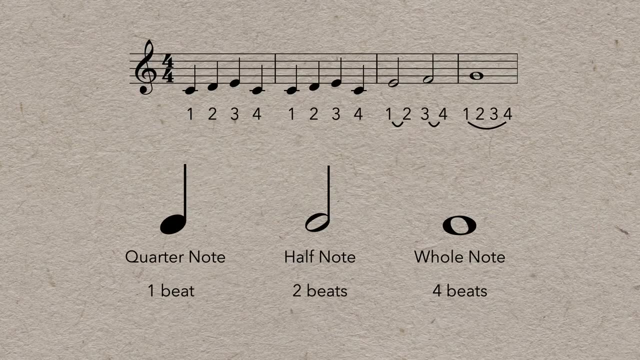 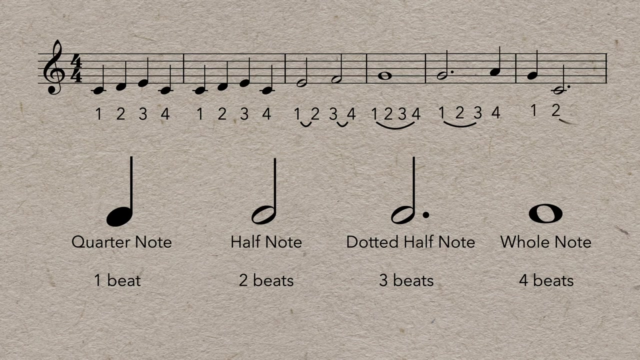 and whole notes which are four beats long. So that gives us options for one, two and four beat notes. And if we want a three beat note, we use a dotted half note. And if there's a different number of beats in the bar, every bar has a different number of beats in it. So if you're 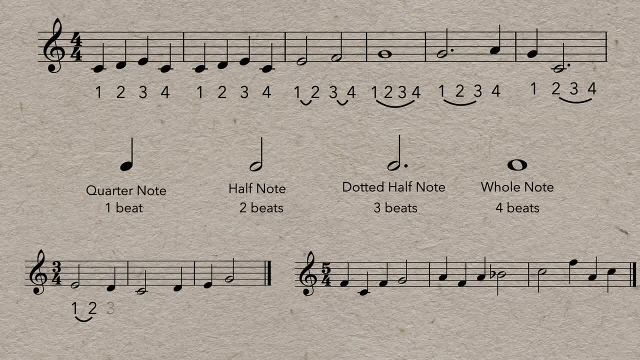 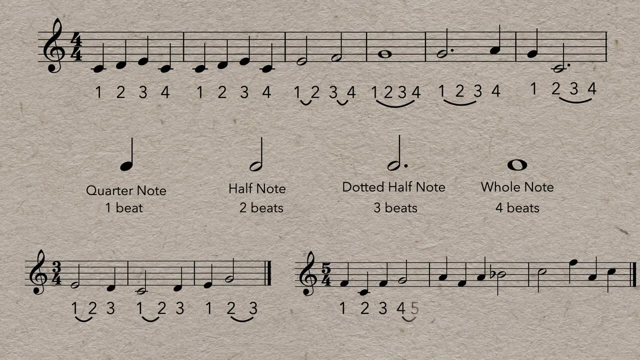 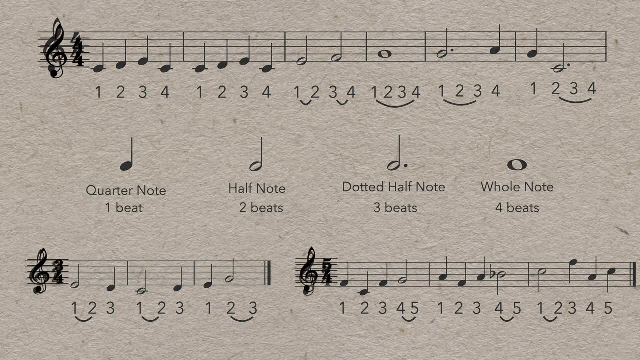 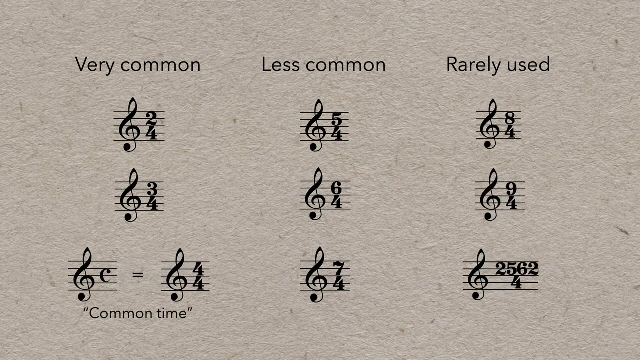 counting four beats in a bar. everything still works out exactly the same way. Any whole number of beats in a bar is possible, but some are more common than others. In fact, 4-4 is so common that it's sometimes called Common Time and it's notated with a C. 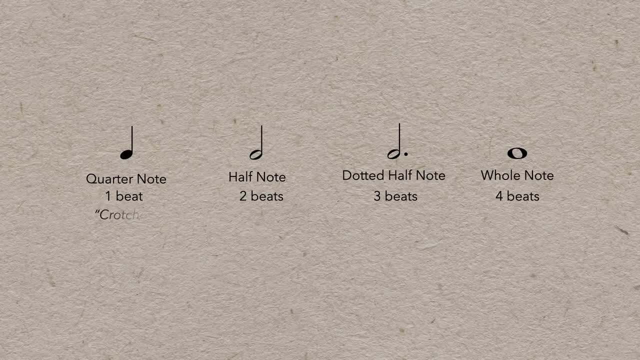 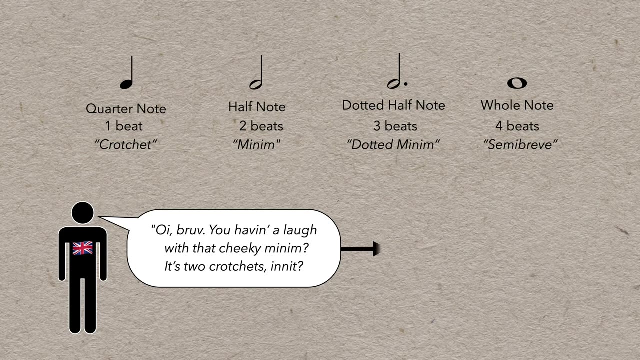 on the staff And speaking of different names, for the same thing, the British have a different set note values, just like they have for a lot of different words. Use whichever one you like, but I'll be using quarter, half and so on, not only because that's what I'm used to. 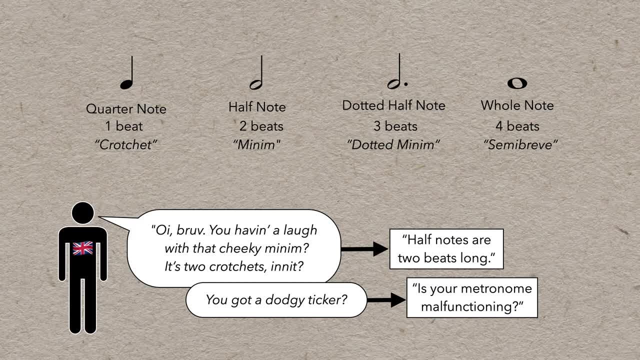 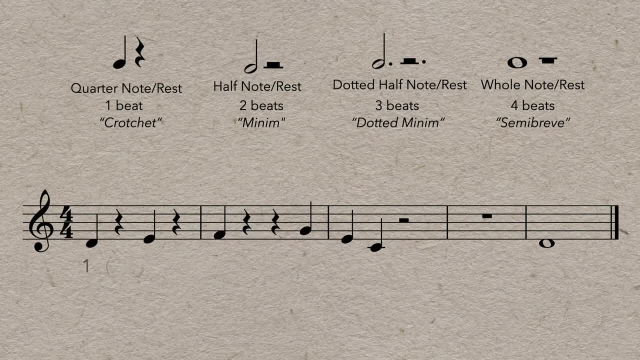 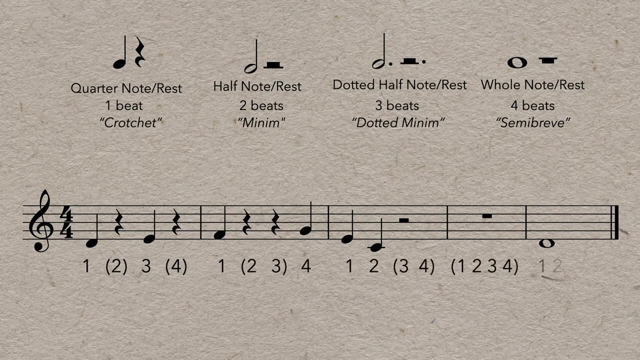 but because I think it makes the rhythmic relationships between note values much clearer. Each one of these notes has a corresponding rest, which just means silence instead of sound for some number of beats. One thing to note is that the whole and the half rest look fairly similar. 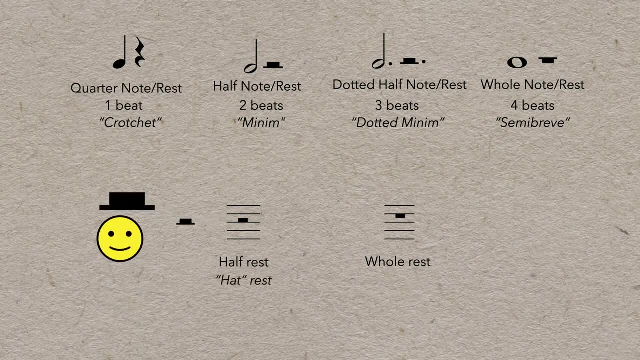 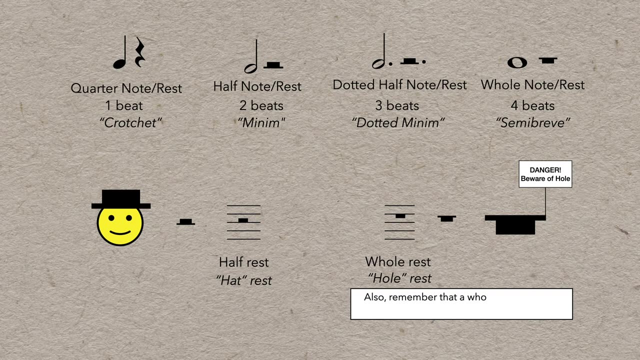 To remember the difference. you might think of the half rest as looking like a hat, The hat rest And the whole rest looks like a hole that you don't want to fall into. The whole rest Also. a whole rest- is four beats long and it hangs down from the fourth line of the staff. 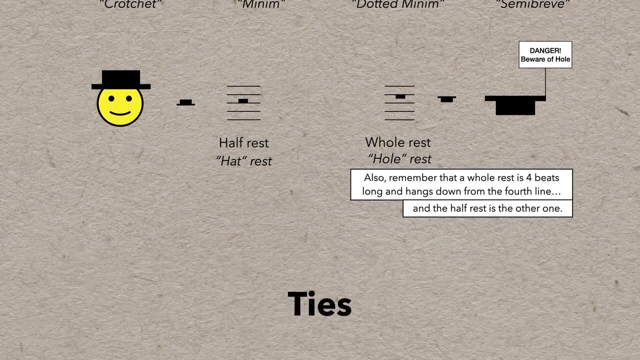 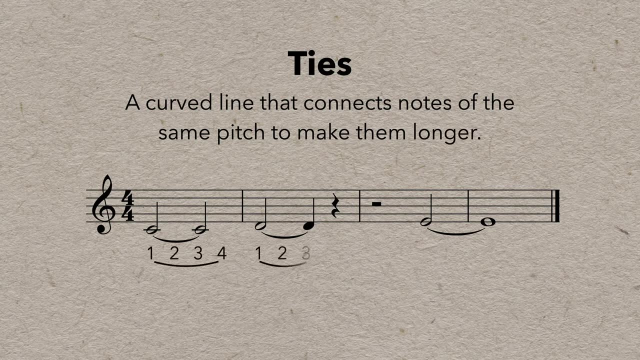 And the half rest is the other one. There's also something called a tie, which is a curved line that connects notes of the same pitch to make them longer. They can occur inside the bar or over the bar line, And that's basically all there is to the bass game. 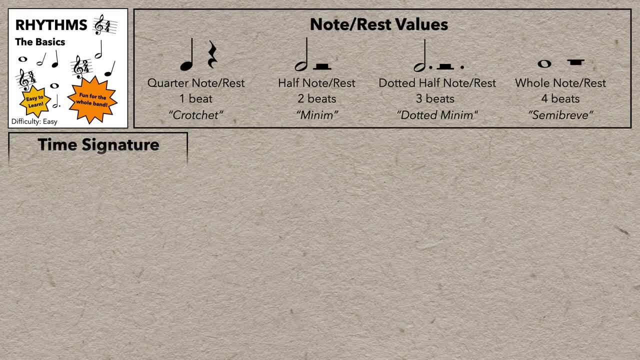 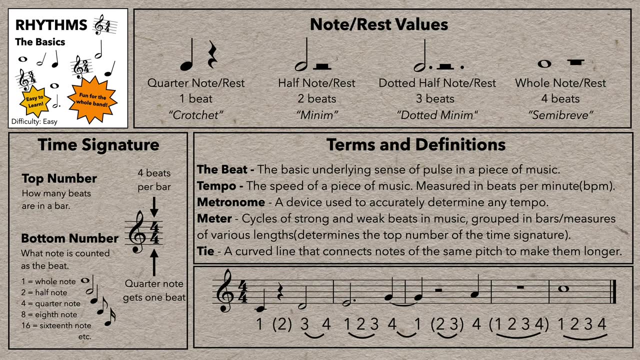 This stuff can take a bit of practice to get used to, but the patterns and rules are all relatively simple, And not only can you play a lot of music with just these rhythmic concepts, it sets you up for understanding everything that's coming next. 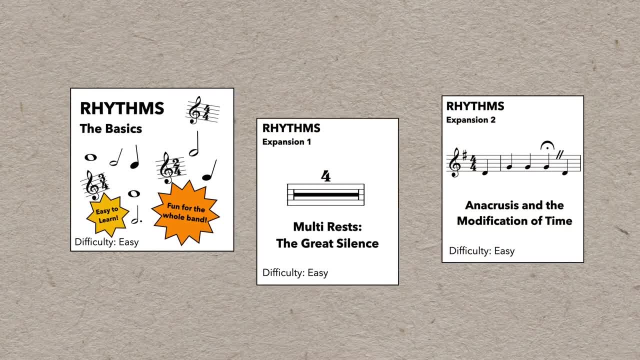 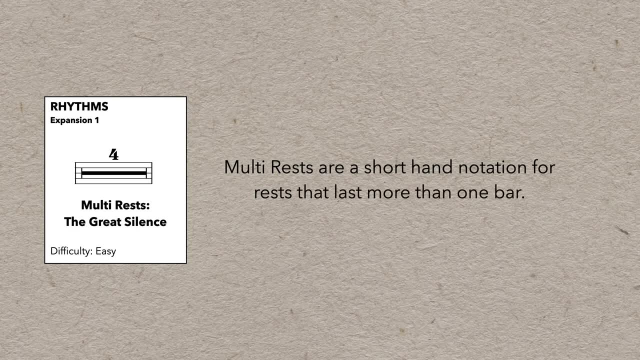 If you're ready to move on, it's time for our first expansion. a small and simple but useful tool: Multirests, The Great Silence. Multirests are a shorthand notation for rests that last more than one bar. This passage has a bunch of bars of rest in a row. 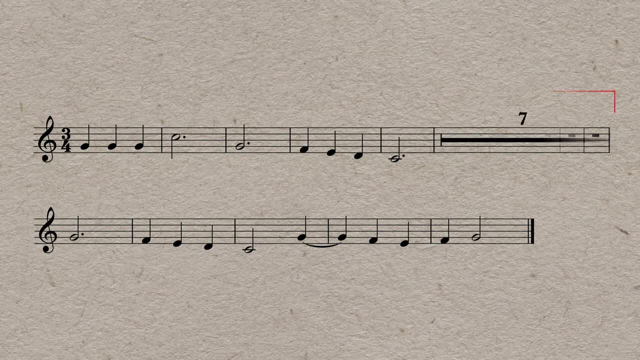 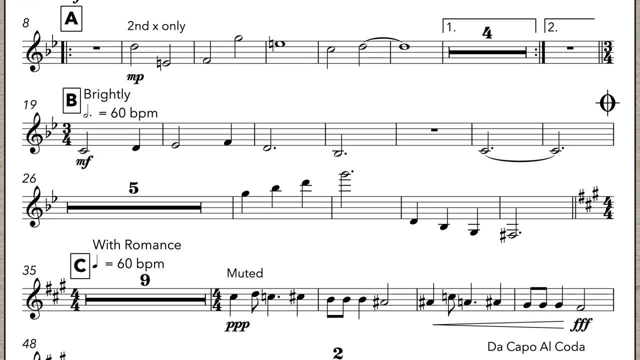 but it's hard to tell how many there are at a glance. But with multirests it's really clear. Multirests mostly show up in longer pieces when you're playing with other instruments. Music might get boring if everybody played all the time, so composers often have different. 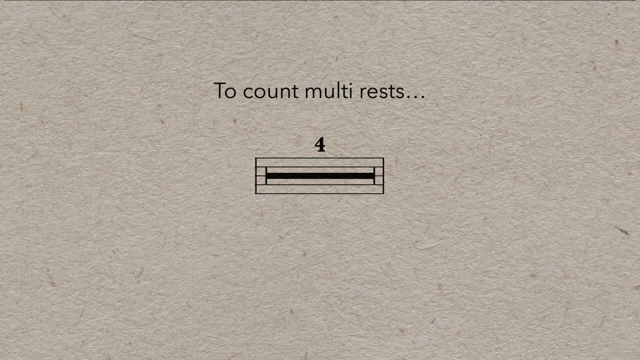 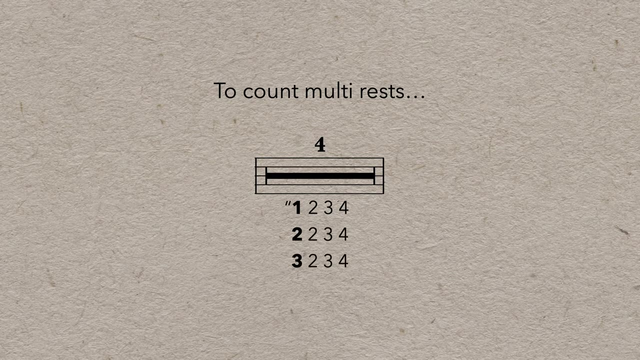 instruments or different sections featured or resting at any given time. We usually count them as 1, 2,, 3, 4,, 2,, 2,, 3,, 4, 3,, 2,, 3,, 4, and so on. 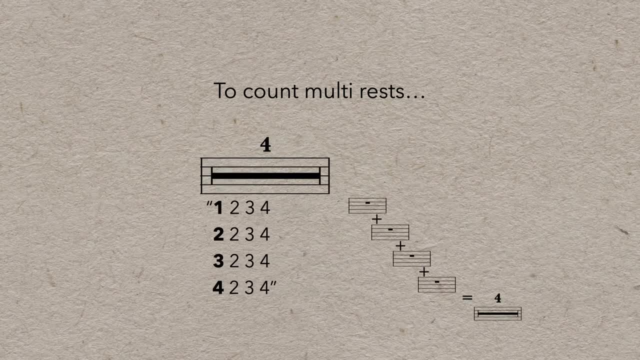 That way you can keep track of how many bars have passed and stay in time with the beat, And don't be afraid to discreetly count on your fingers so you don't get lost. It can be pretty easy to zone out and forget what bar you're on. 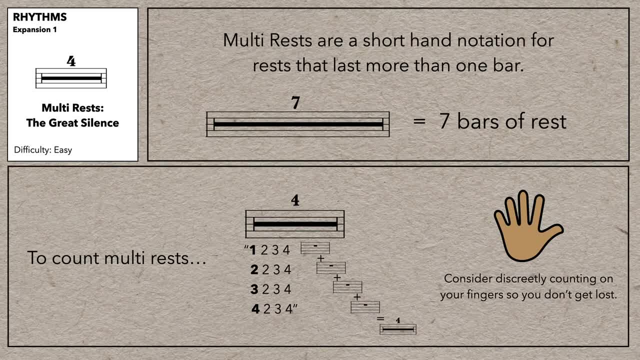 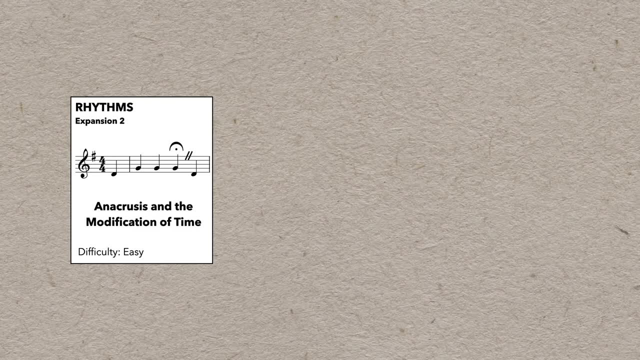 That's Multirests, just a quick mini-expansion to build on what we already know about rhythms. The next expansion of this game is called Anacrusis and the Modification of Time. Now, that may sound like the title of a fantasy novel, but Anacrusis is a fancy. 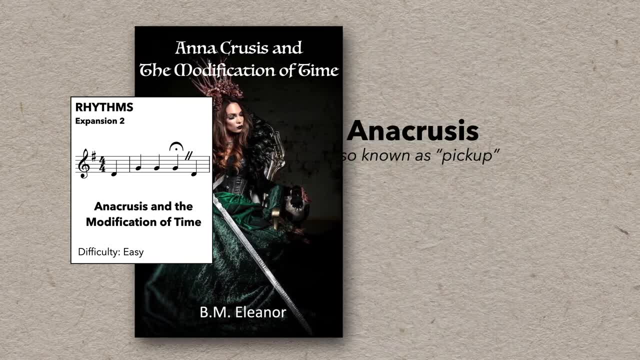 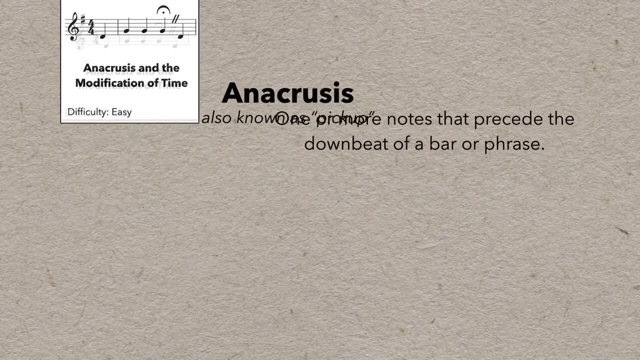 name for a really simple thing. It's probably more commonly known as a pickup note or pickup beat. It occurs when one or more notes precede the downbeat of a bar or phrase, and it's something you've probably been doing since you were little. 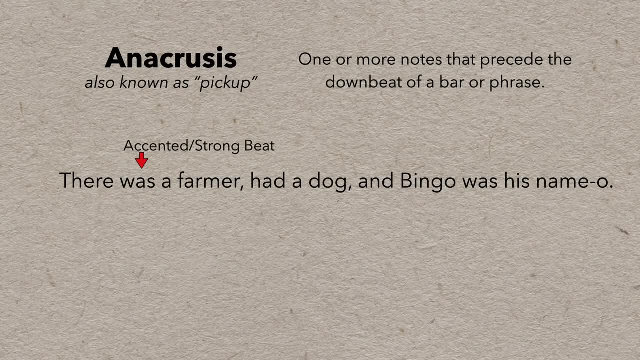 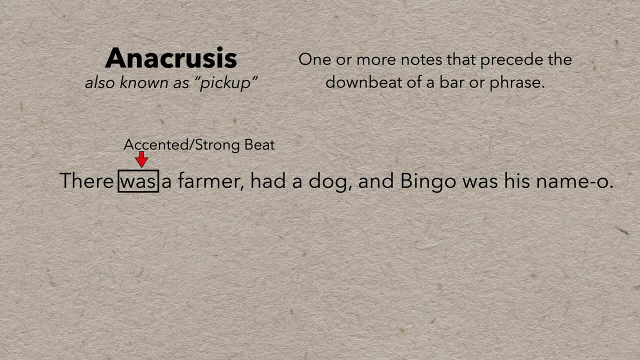 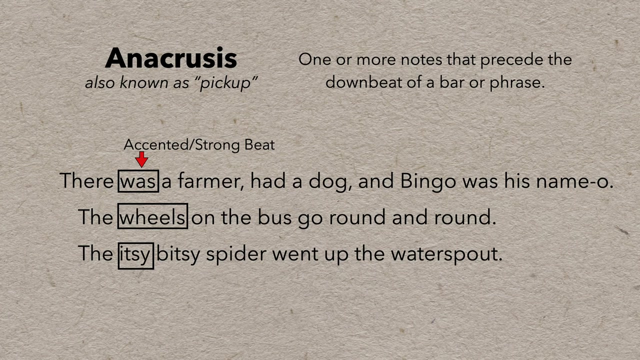 You might remember the song Bingo. The accented strong beat doesn't happen on the first word, It happens on the second And it works the same with the wheels on the bus And the itsy bitsy spider. The notes before the strong beat are the pickup or the anacrusis. Looking at these songs in 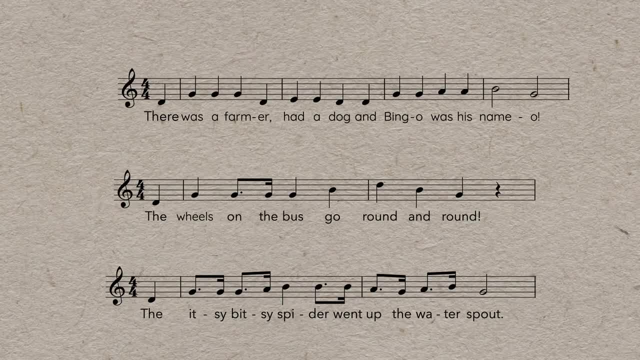 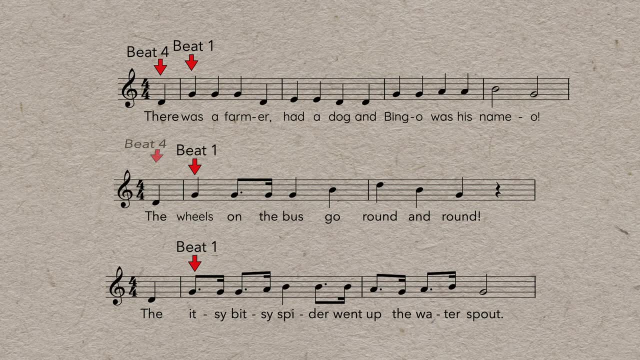 notation. you'll see a little preview of the rhythms that are coming up in the next video, But all you really need to know is how to play them. If you want to learn how to play them, please keep watching If you're playing music with other people. 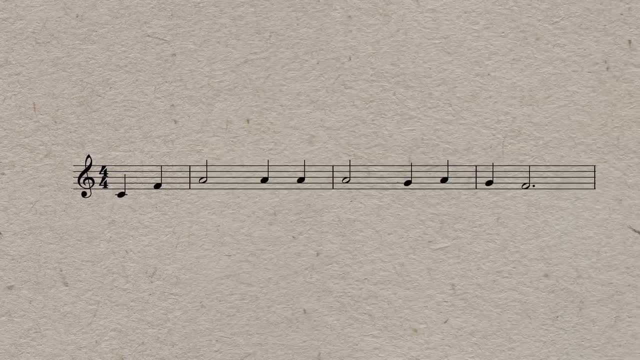 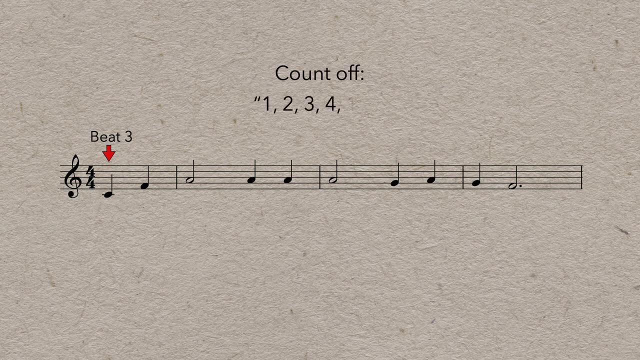 you want to make sure that you're all starting at the same place or it can get really messy Here. you start on beat three, so you might hear a count off or a bar with two beats, Something like 1, 2, 3, 4, 1, 2.